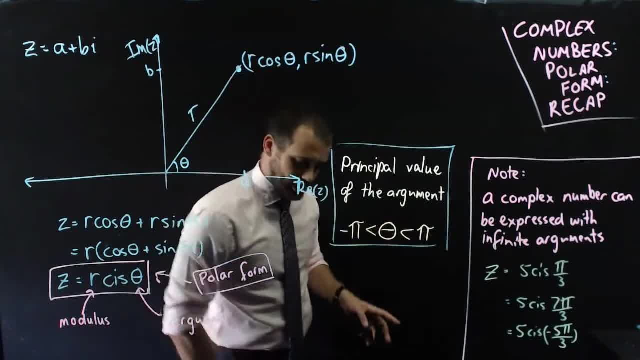 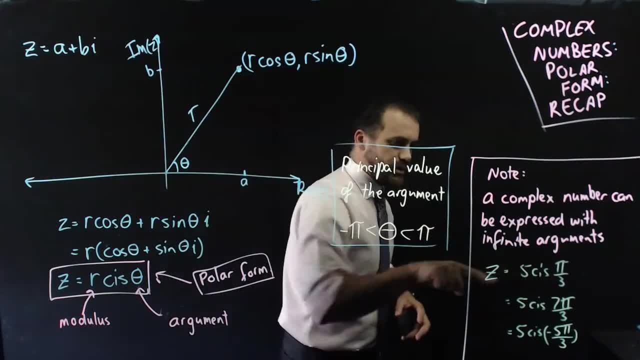 pi and down to negative pi. That's most polite. So out of these three versions here only one uses the principal value of the argument, and it's that one. So a quick example. here we're going to convert Cartesian form to polar form: z equals 4 minus. 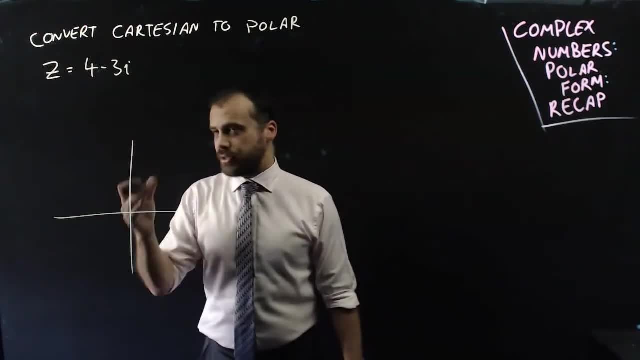 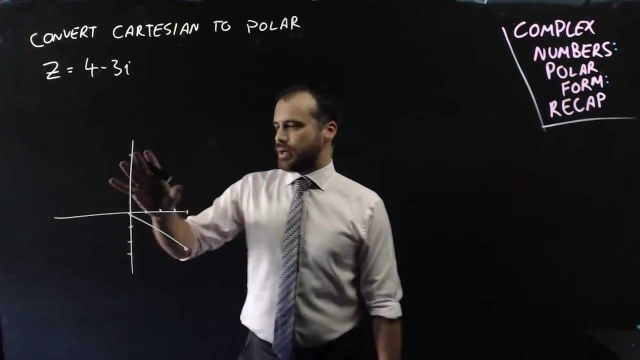 3i. if I drew it on a Cartesian plane or an Argand diagram- sorry, it would look like 1, 2, 3, 4,, 1, 2, 3 down here somewhere- Now I can find the r-value because I know Pythagoras'. 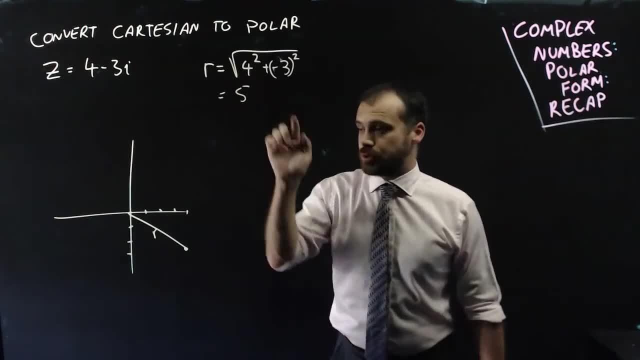 theorem, The square root of 4 squared plus negative 3 squared is equal to 5.. So that r-value is 5.. Now I just need to find the square root of 4 squared plus negative 3 squared. Now I just need to find the square root of 4 squared plus negative 3 squared, So that 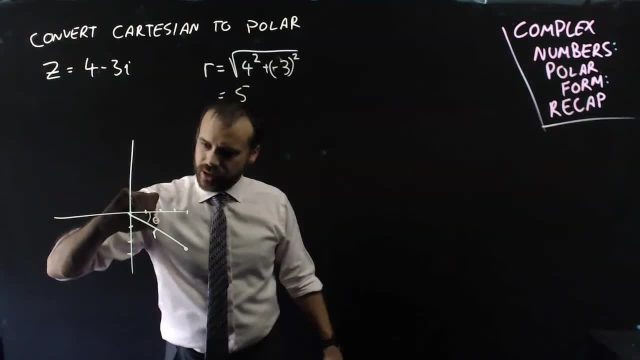 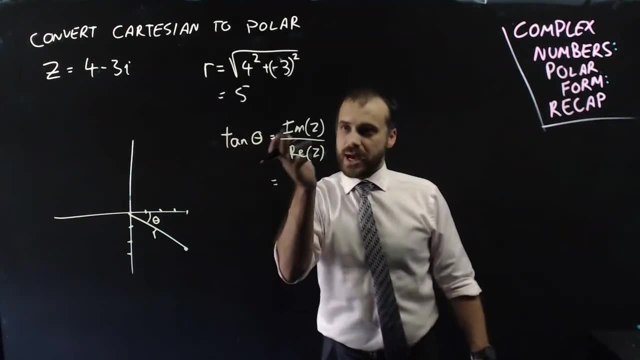 r-value is 5.. Now I just need to find the square root of 4 squared plus negative 3 squared. So I need to find this angle here and it's going to be negative, Alright. so if I need to find that angle, it's the same every time: 10 theta equals the imaginary component over. 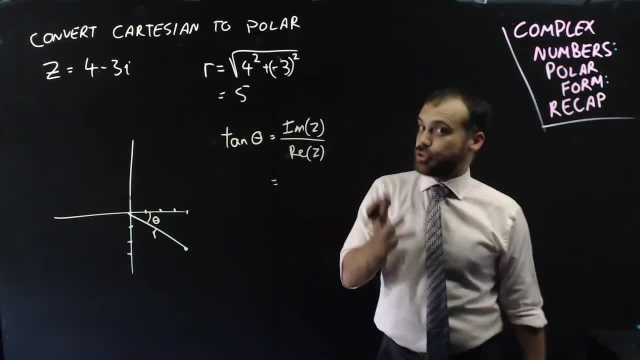 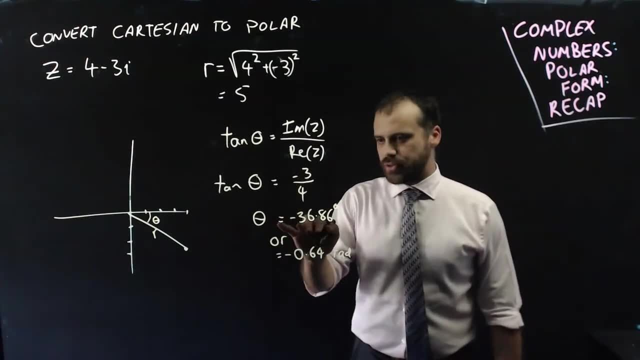 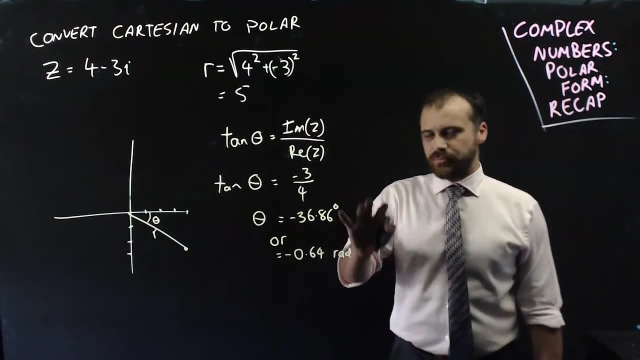 the real component and then adjust for whatever quadrant you're in. Now, if the numbers were neat I'd do this calculator free, but they're not neat, So I put that into my calculator and I get negative 36.86 degrees or negative 0.64 radians Depending on what mode your 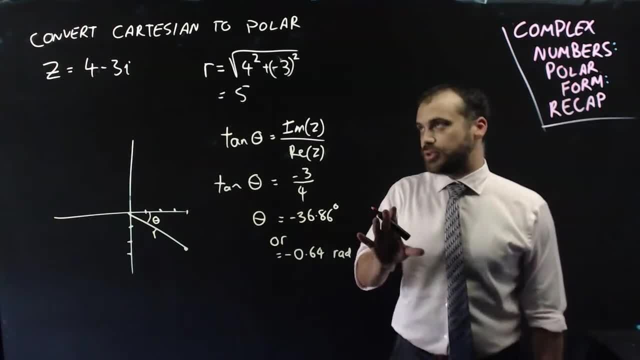 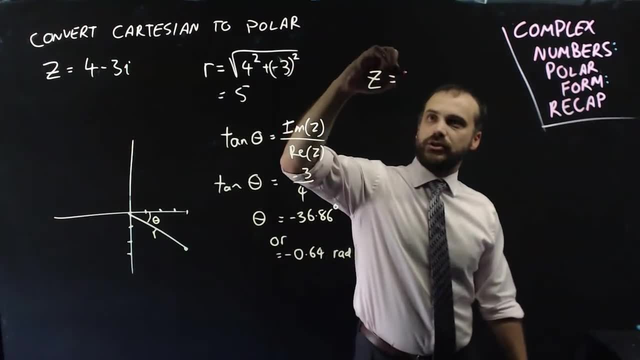 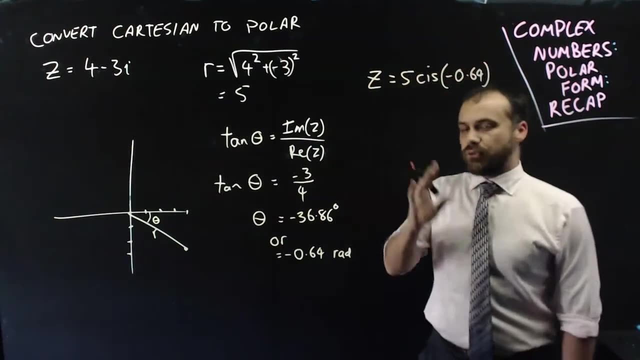 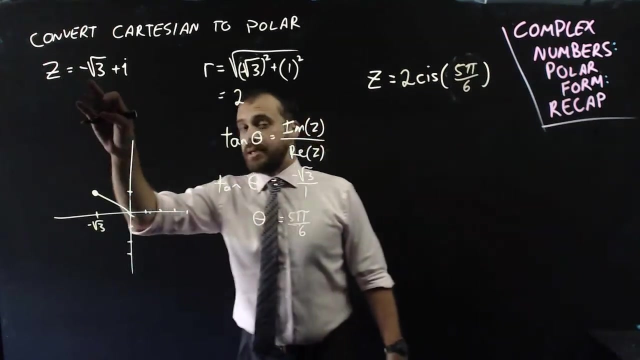 calculator is in, in, and what's being asked of you all? right, so we can finally give this z in polar form. it's equal to five cis, and let's put it in radians: negative zero point six, four. and just to give you another quick, very super duper quick example, if the complex number had been different, say negative, 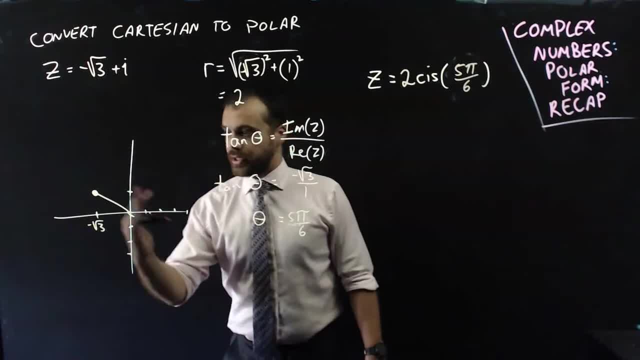 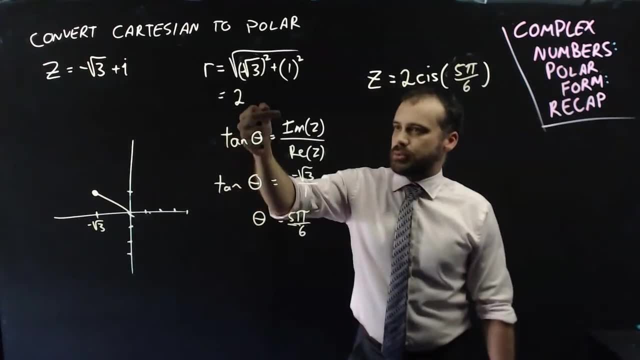 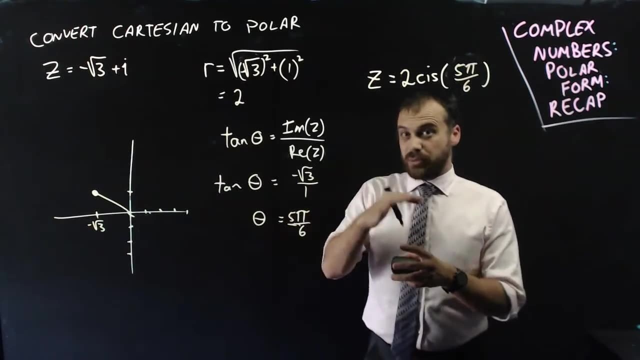 root three plus i. we could draw it on a cartesian plane like that in our second quadrant we could find the modulus of two tan. theta equals imaginary over real, which gives us this value here. now, if you're working on your head, you'll figure out that theta is equal to pi on six as the reference angle. 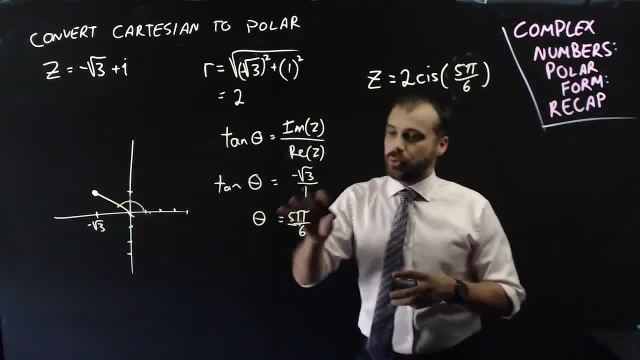 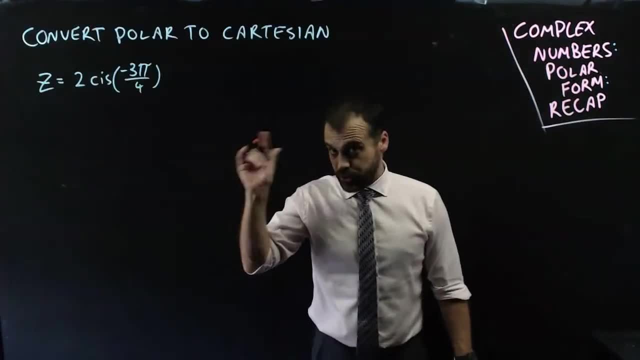 but you don't want the reference angle. you want this angle, which would be five pi on six, and that would be that, but in polar form. now what if you want to get the square root of negative zero point six and you want to go the other way? well, it's a good idea to keep in mind what this actually is. 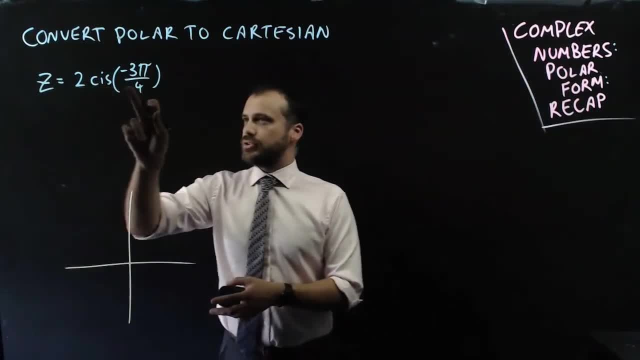 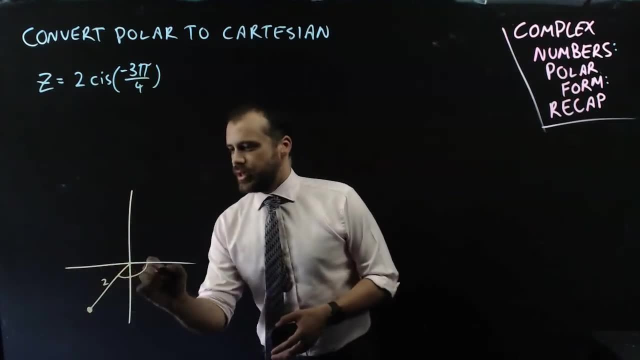 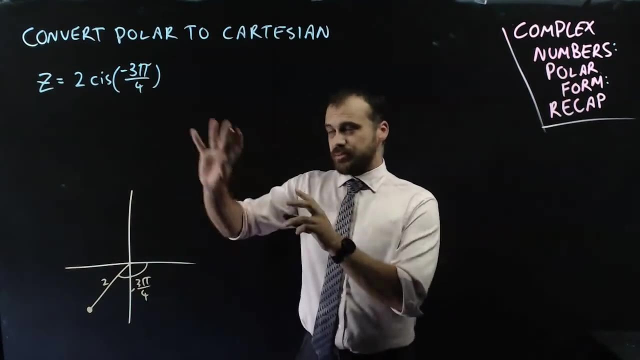 remember argand diagram: length of two. angle of negative three pi on four. so it looks like this: a length of two. we're looking for that coordinate right there and that angle is negative three pi on four. the other thing that makes this pretty straightforward is remembering what cis actually. 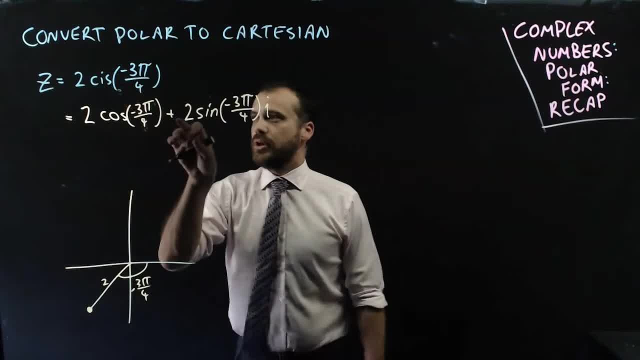 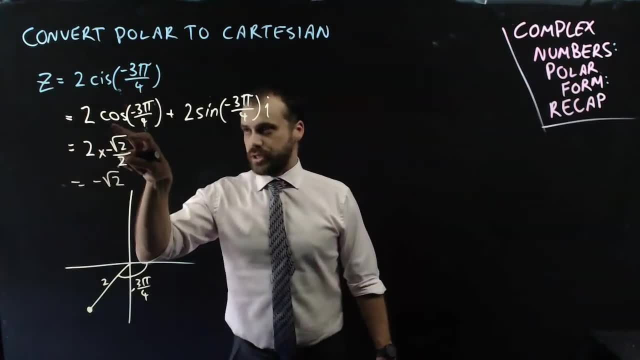 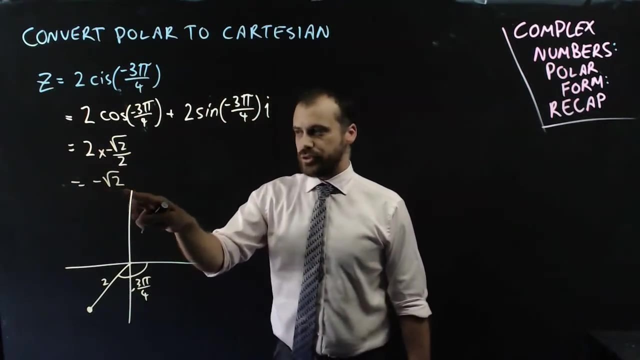 means it's short for 2 cos that angle plus two sine that angle, i. so as long as you can solve that, which you should be able to do, cos negative three. pi on four is the same as negative root two on two, which means that that is negative root two. now that's our real component of z, and of course you should also be able to solve: 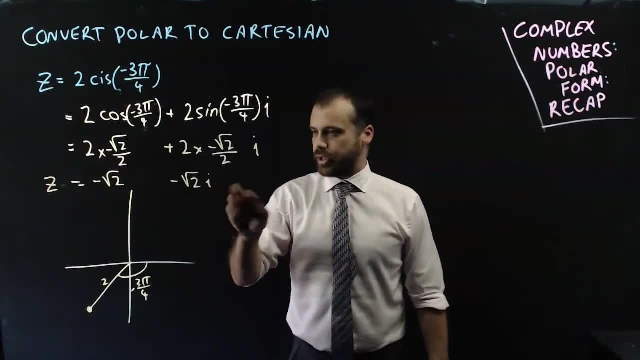 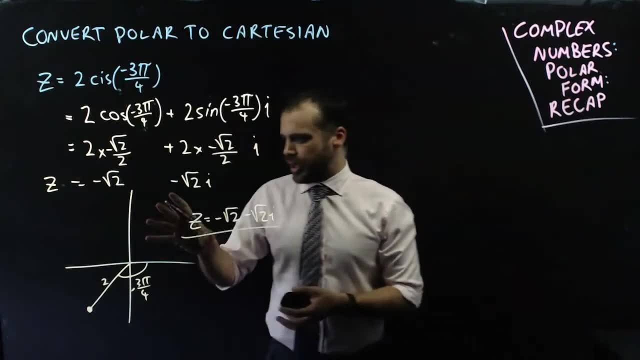 that relatively straightforward minus root two, i, and that's our neat little answer there. now you don't have to draw the argand diagram, but i think you'd be a fool not to, just because you can double check to make sure this makes sense. this makes sense for a couple. 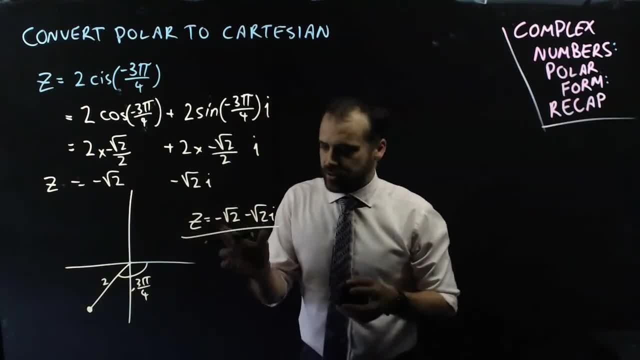 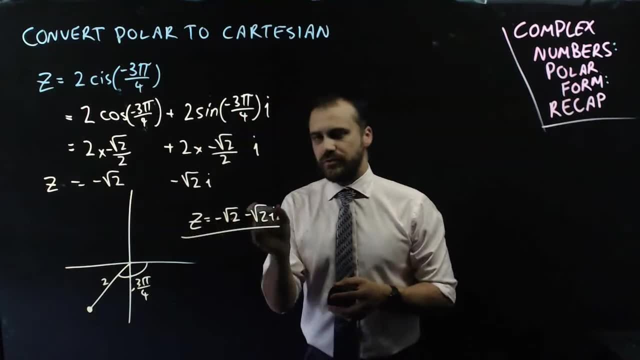 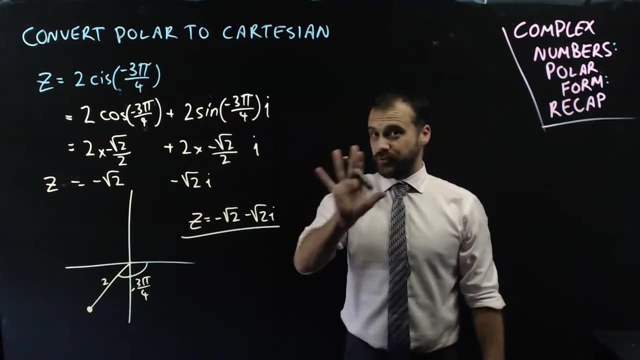 of reasons, we've drawn it in the third quadrant, so these should both be negative. also, this angle here ends up being 45 degrees, right, so we would expect those two values to be the same. so that's converting polar to cartesian, and being able to do this is really important for one simple reason. 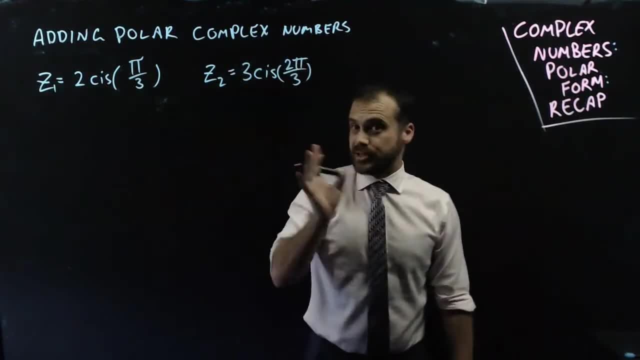 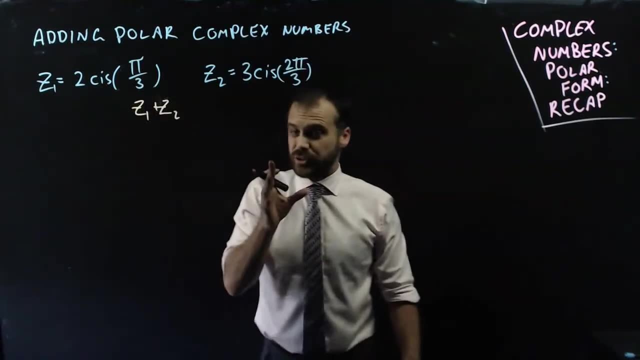 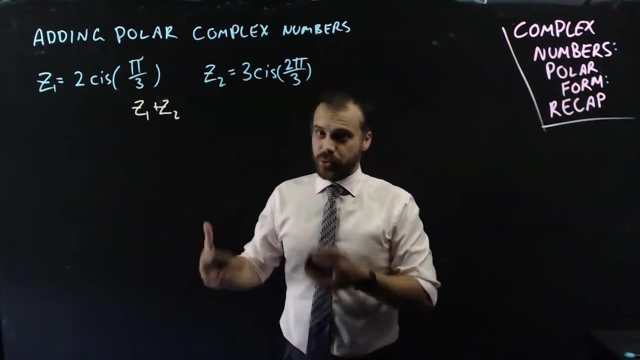 there is no easy way of adding polar complex numbers. if you want to add complex numbers, that is z1 plus z2. you don't have a choice here. you need to convert them to cartesian form, add them together in cartesian form and then, if you want them in polar form, put them back again. 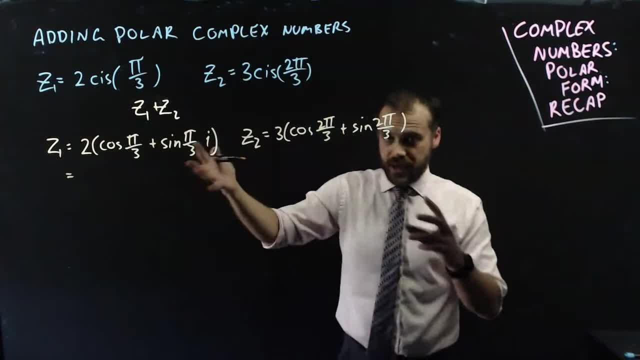 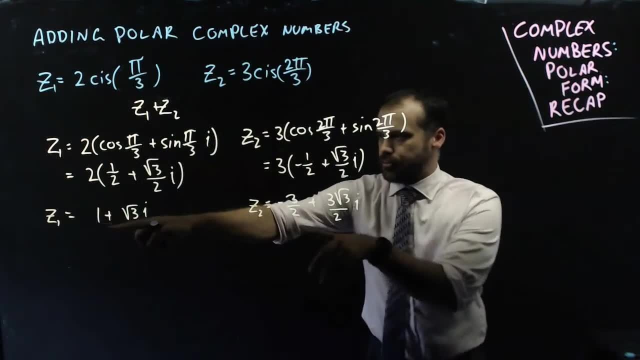 so we take them in cis form and convert them to the expanded version of cis and with a little bit of work you'll get them into cartesian form. and adding them is really simple. add your real components, add your imaginary components, which gives us a final answer of this. now, if they 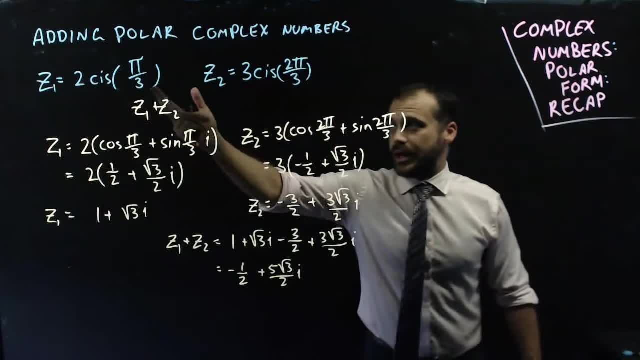 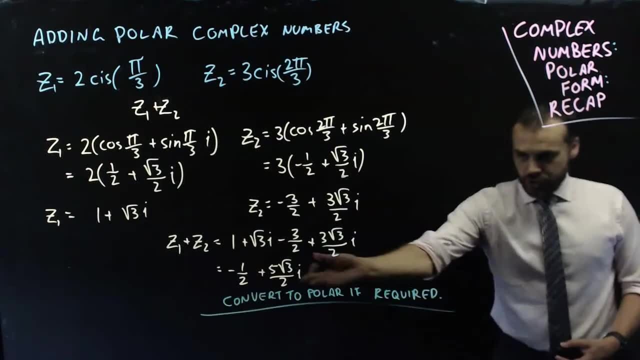 wanted it back in polar form, they would have to convert them to cartesian form and add them to polar form- which is likely because they gave those two in polar form- then you would then need to convert that and i've already shown you how to do that, so i'm not going to do it right now. convert- 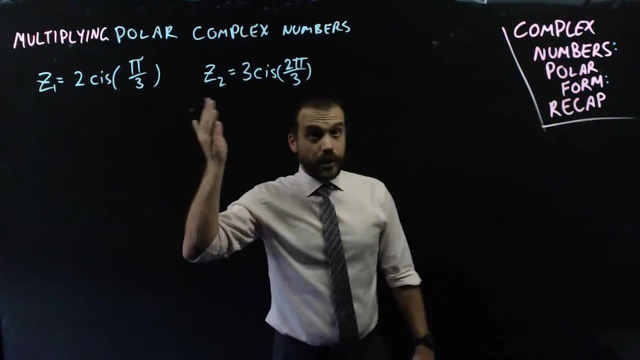 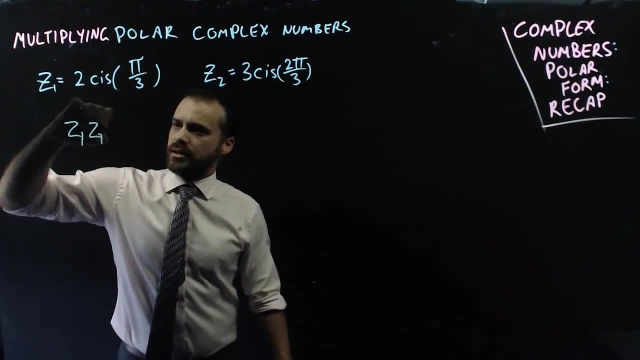 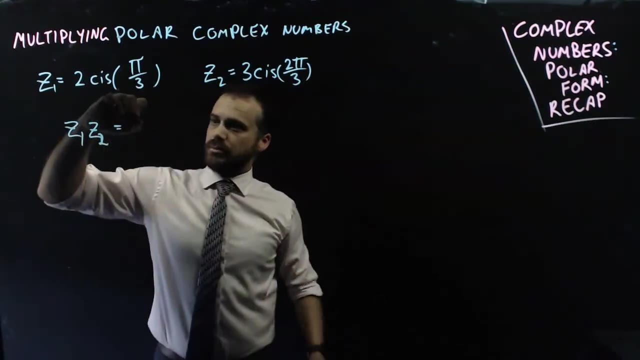 to polar if required. now, different story if you are multiplying polar complex numbers- and it's way easier to do so if we're doing z1, z2 and we're multiplying these two together. all we need to do is take these two numbers and multiply them together, and then 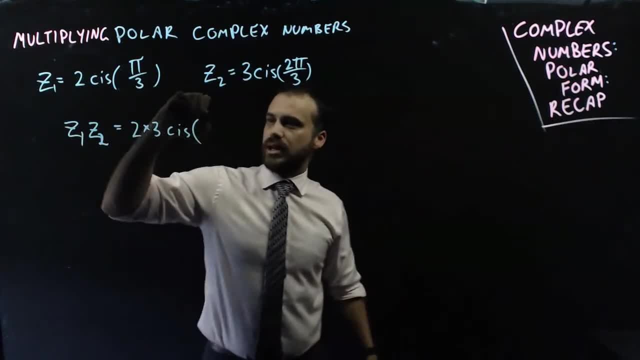 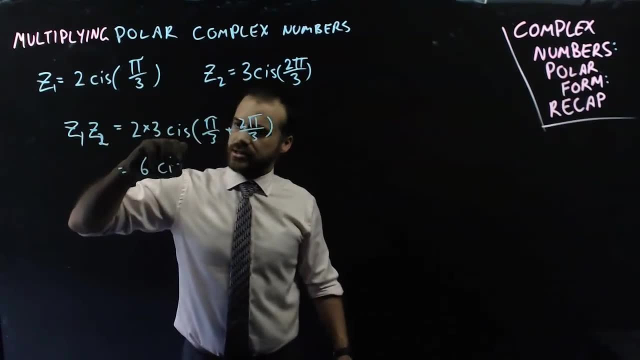 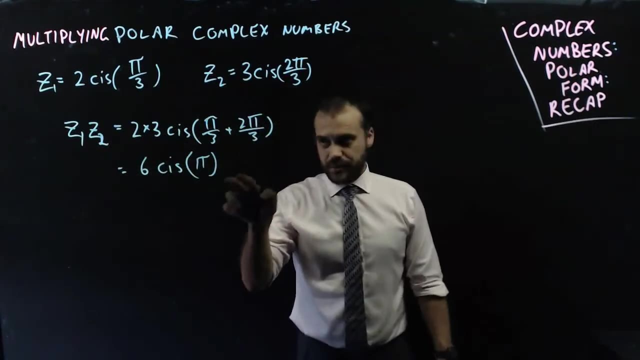 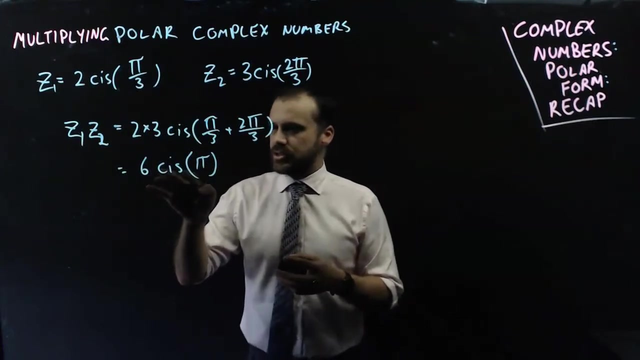 add up the whole functional learning a little bit. so let's go with this and then add our angles together: pie on three plus two pi on three, we'll get an answer of six cis, uh, three pi on three, which is pi, and that seems special. it's special because pi, 180 degrees, is on the x axis. now, if you 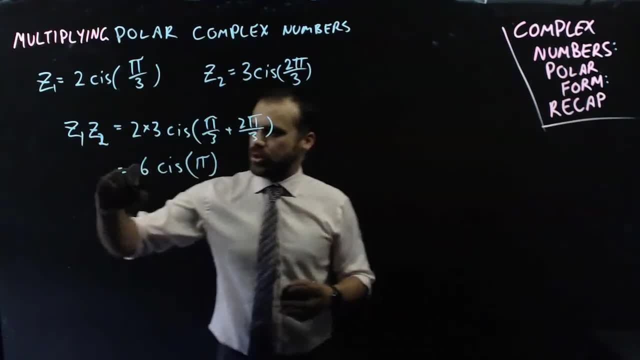 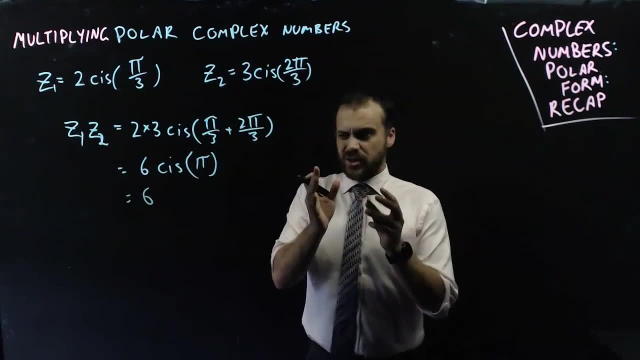 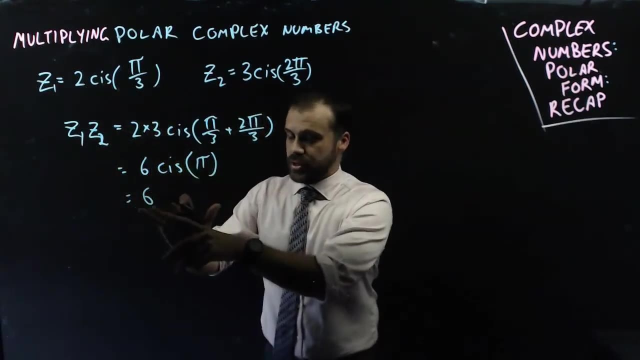 think about what cis is again. it's six cos pi, that's six times one, so we get six as a real component. And then it's 6 sin pi i, 6 sin pi 0, so 0 i. That means that if you multiply these two complex numbers together, you get this answer, which is purely real. 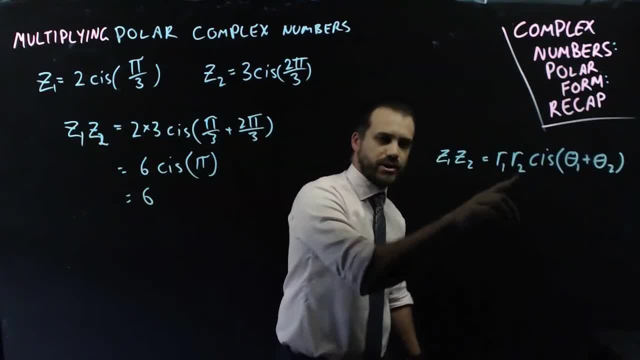 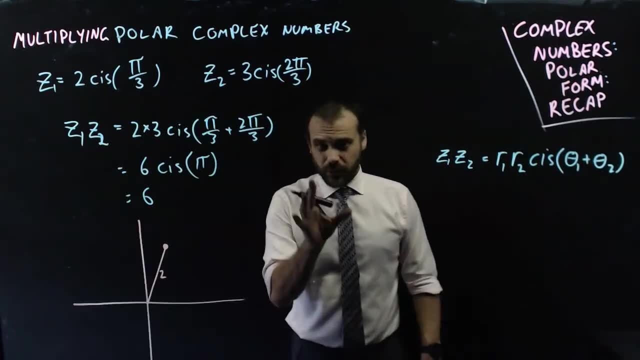 Now I really just need to tell you the formula: z1 times z2 equals r1 times r2, cis theta1 plus theta2.. And we've got something special or similar for division. But before I get there, I want to talk to you about the geometric interpretation of multiplying complex numbers. 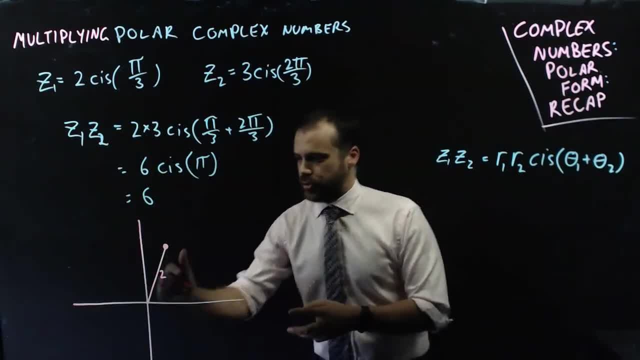 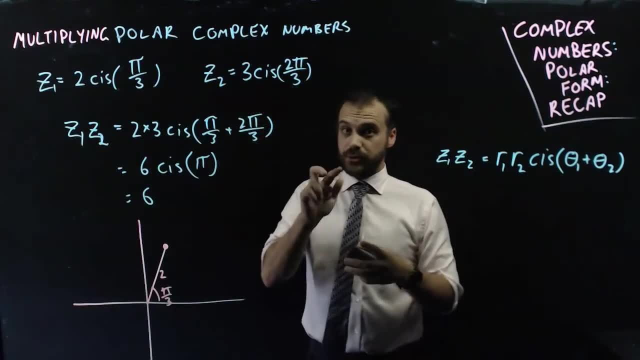 This one here is z1, 2 cis pi on 3.. That angle, there is pi on 3.. Now, when I multiply by 3 cis 2, pi on 3, I'm doing two things. One, I'm scaling it up. 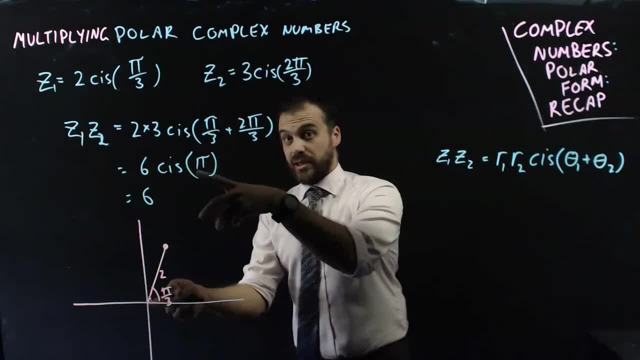 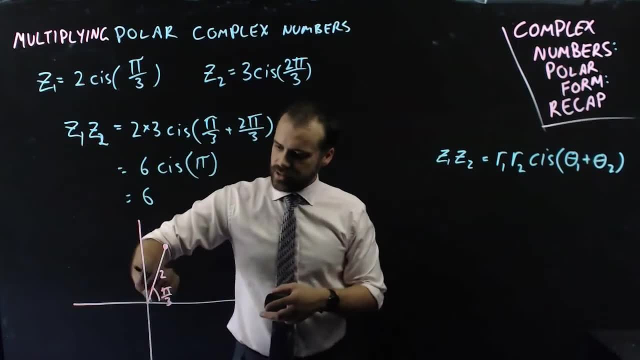 Because, remember, I took the number 2 and multiplied it by 3, and we get the length of 6.. What I'm also doing is adding the angle 2 pi on 3.. Which has the, Which has the effect of taking this angle here and adding 2 pi on 3 to it. 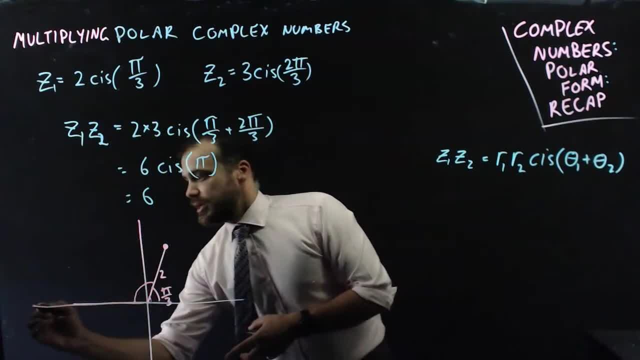 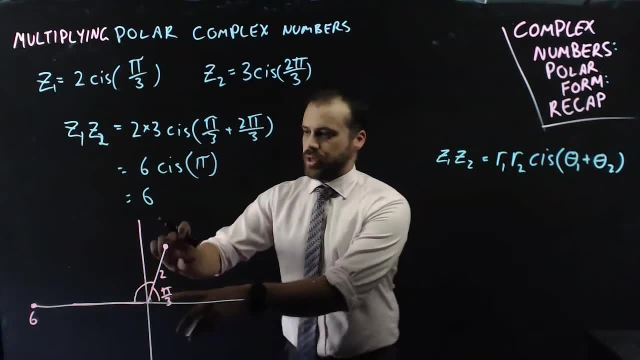 So we get something that rotates and scales up. So this was z1, 2, cis pi on 3. We've rotated it and scaled it up, Or vice versa, scaled it up and rotated it. Same idea. Let's do division. 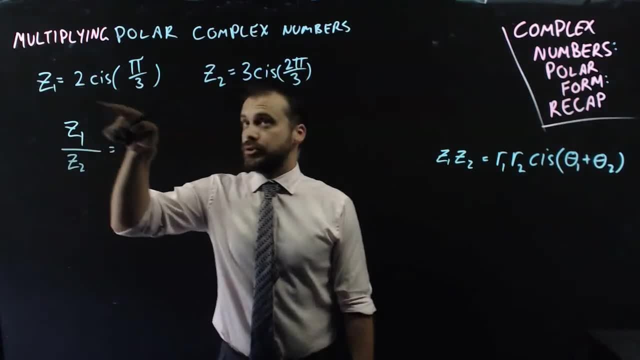 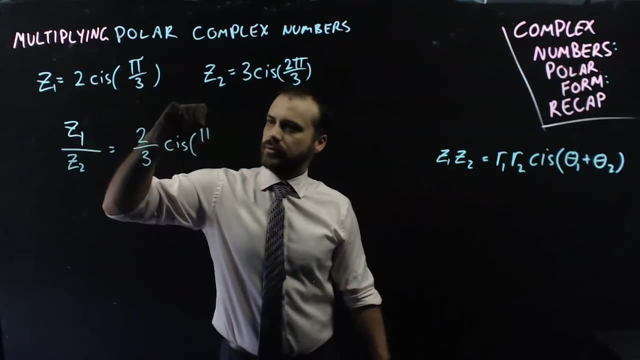 Now this is going to work just how you'd expect it to as well: 2 divided by 3, so our r's divided by each other, And then cis, Angle, Minus angle, And of course we should clean that up a bit. 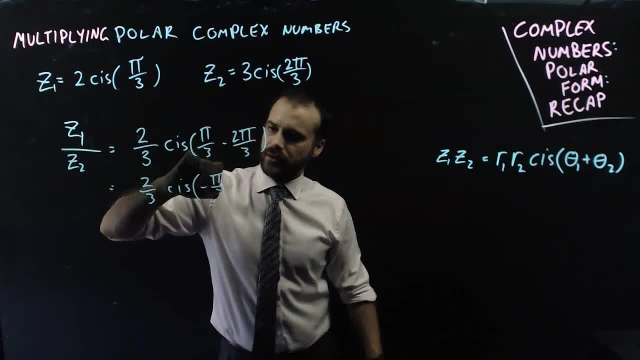 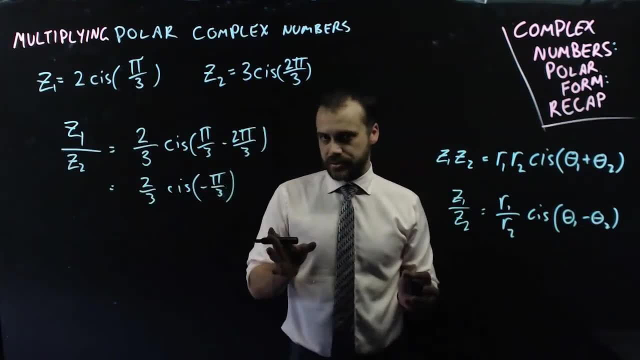 2, pi on 3, cis negative pi on 3.. A formula right here, Alright. lastly, we're going to look at powers, So raising polar complex numbers to a power de Moivre's theorem- I don't know how to say that. 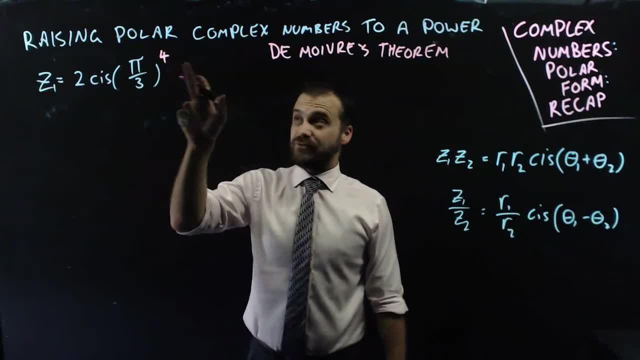 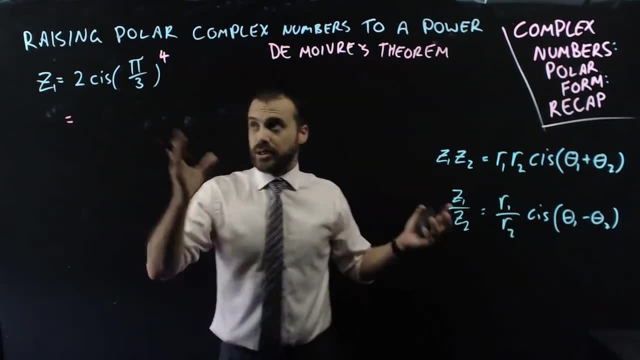 Zen 1 equals 2 cis pi on 3 to the power of 4.. To the power of 4 is just- It's just repeated multiplication, so it works the same. You could work this out just by doing this 4 times, or we can do it faster. 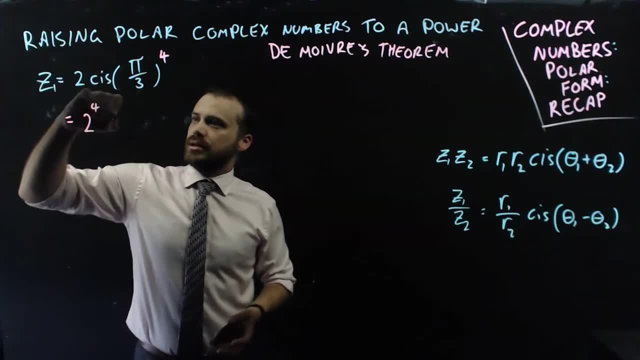 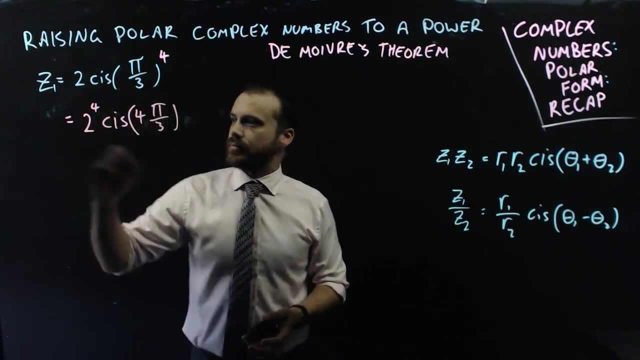 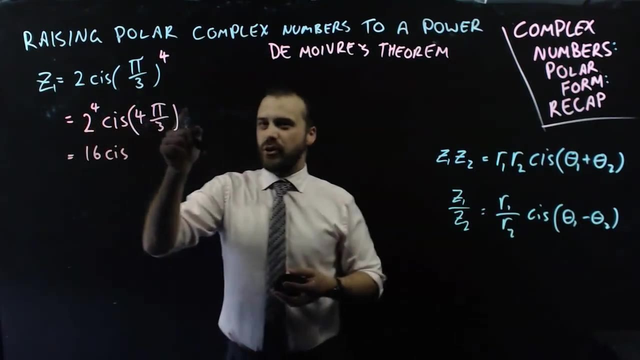 It's going to be this to the power of this cis this times. that, Okay, and tidying this up a little bit: 2 to the 4 is 2, 4, 8, 16.. Cis: 4 pi on 3.. 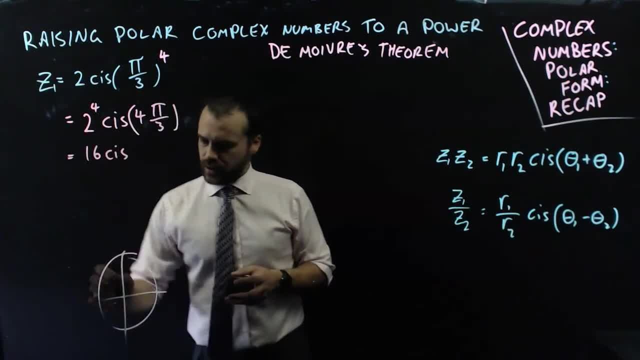 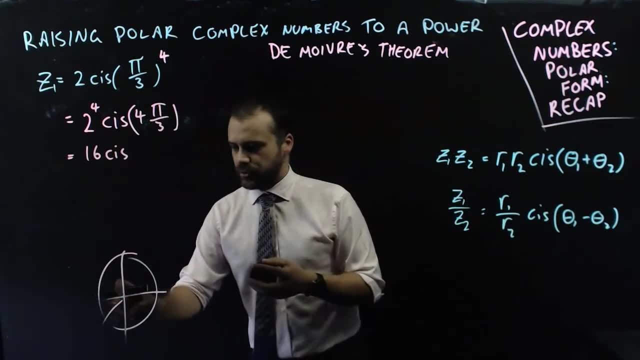 Now 4 pi on 3. Is like over here, But it's not very like polite to express a polar complex number as 4 pi on 3.. So we should express it this way instead: as negative 2 pi on 3.. 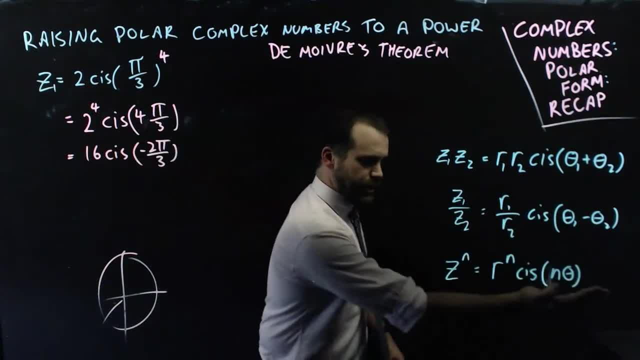 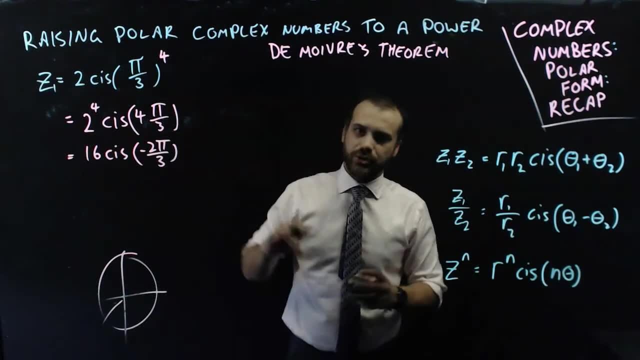 Now, of course, you'll want de Moivre's formula, which is a little something like this: Z to the n equals, r to the n, cis n theta, And then tidy it up. make sure that you're being polite with your argument there. 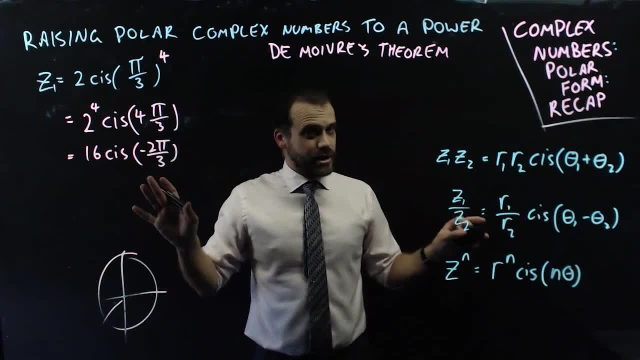 Complex numbers- polar form. That's the full recap. Now let's learn some new stuff. 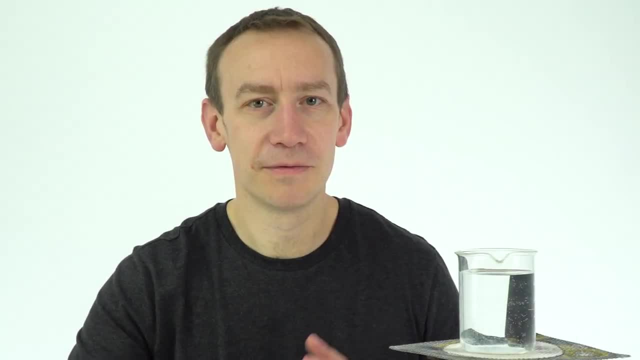 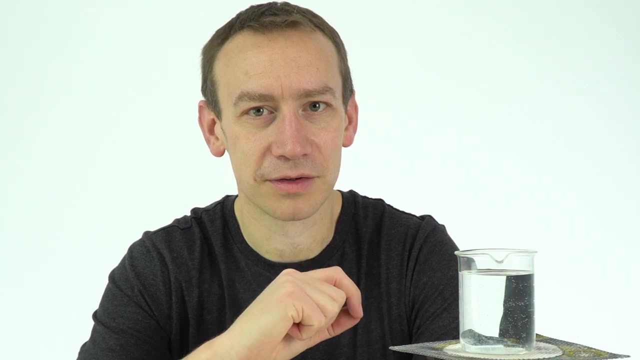 Convection is a method of heat transfer in fluids, so it could be in gases like the air or it could be in liquids like the water. here and in this experiment we're going to have a look at some convection currents. So the setup is just a heatproof mat down. here. I've got a tripod. 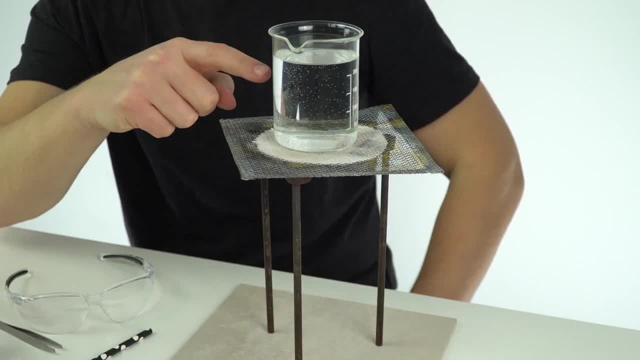 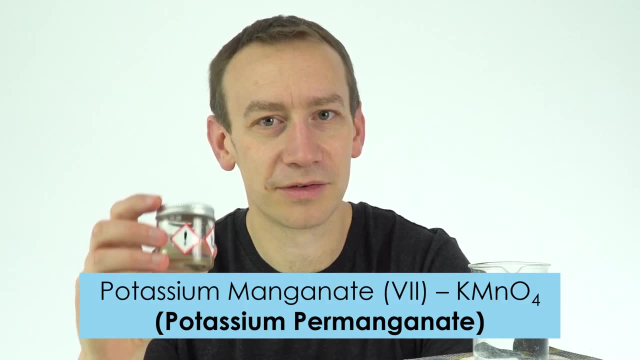 a gauze on top, and then I've got a beaker that's full of cold water. I also have my Bunsen burner in order to heat it up, and we also have this chemical here called potassium manganate 7, sometimes also known as potassium permanganate, and all this is doing is it's acting as a dye.